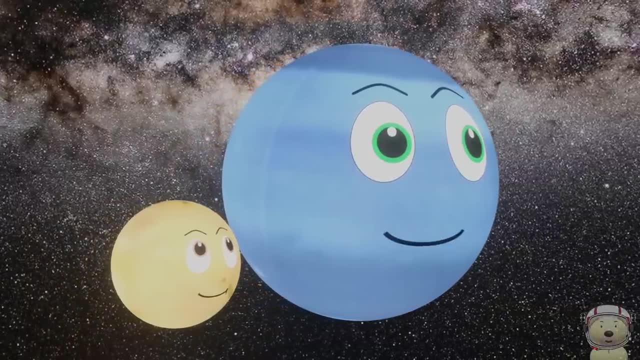 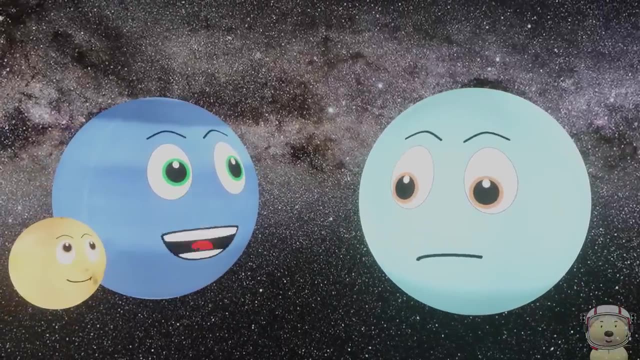 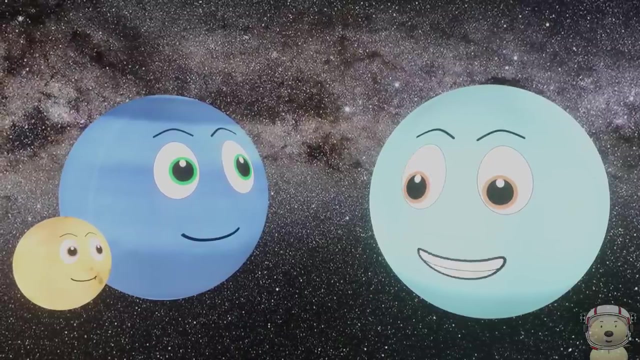 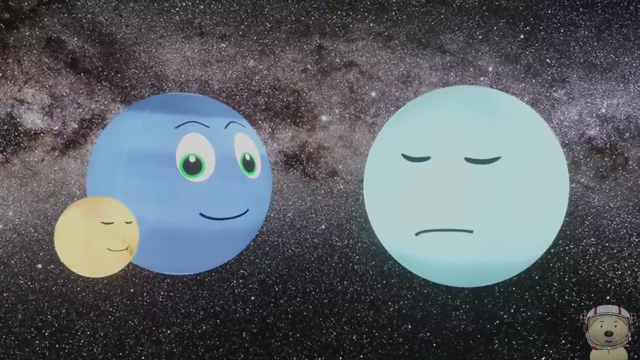 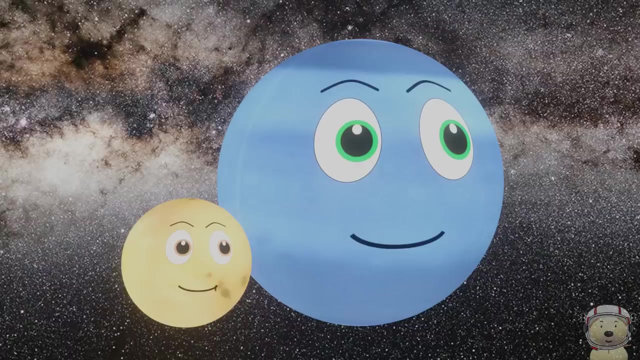 Oh, you heard the song? Yeah, Uranus, my closest neighbour and my closest friend. How are you? What do you want? Have you changed colour slightly? It really suits? you. Stop that. You definitely want something. Wow, now you mention it. 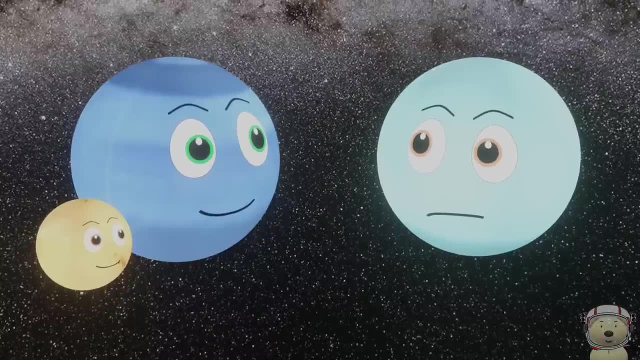 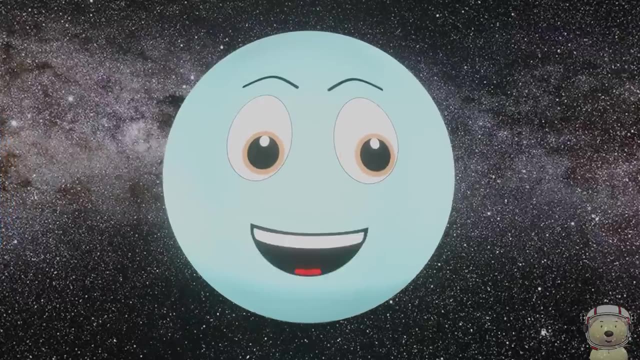 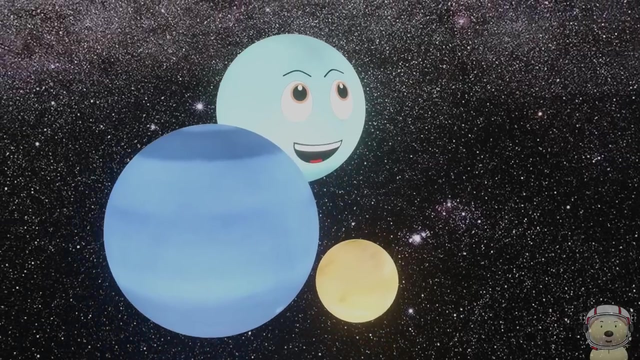 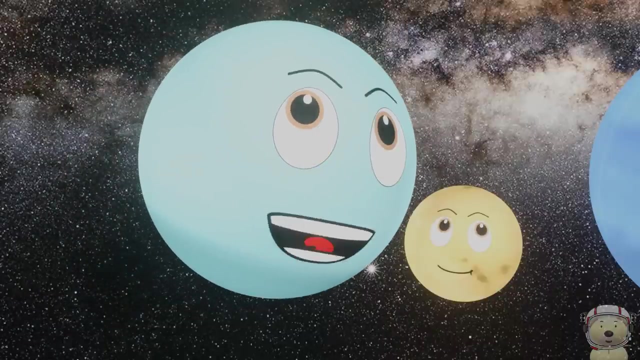 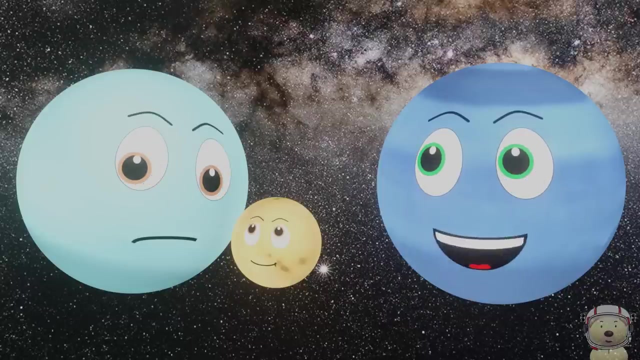 I knew it. We need to get Earth off the computer. He's playing it all day. Ah well, I can definitely help with that, You can. Yes, You've come to the right guest giant. The others have rubbish ideas. Uh, I am literally stood here. 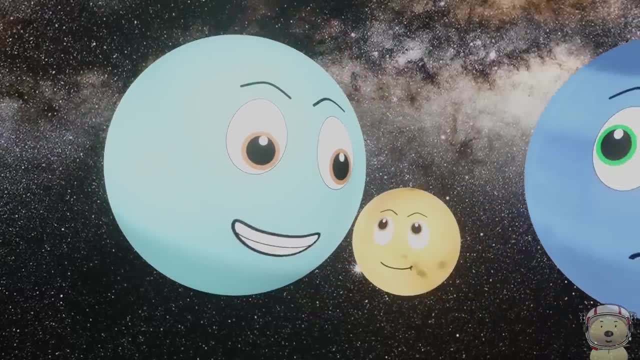 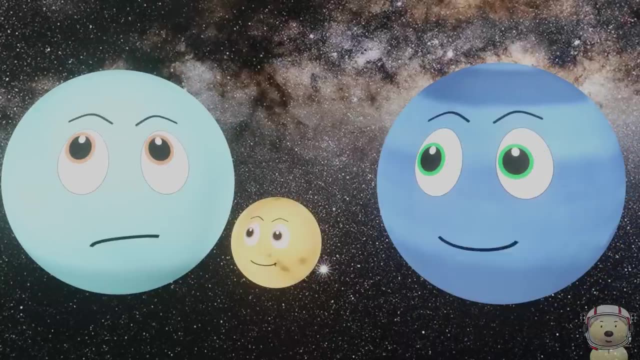 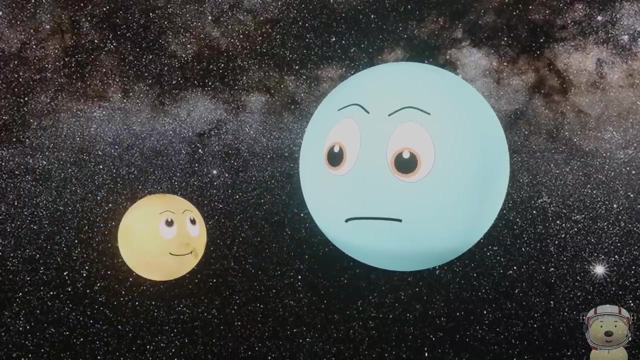 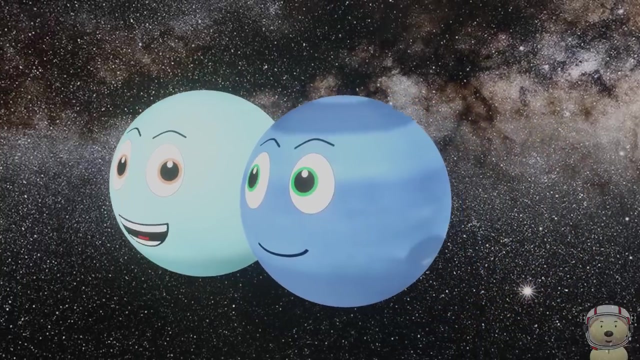 I am the best guest giant in the entire solar system. Hello, Can anyone see me? Excellent, Let's go and get Jupiter, Saturn and Mars. I'm sure they will have ideas. No need I have the best solution to your problem. 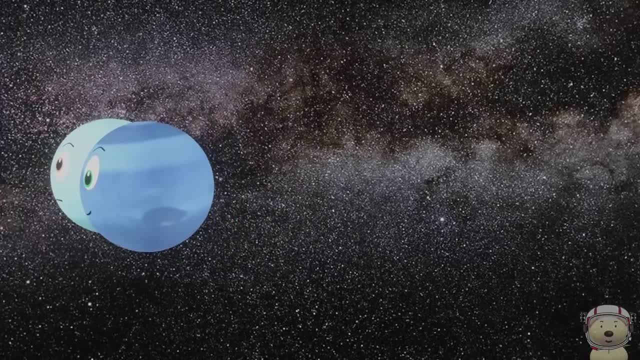 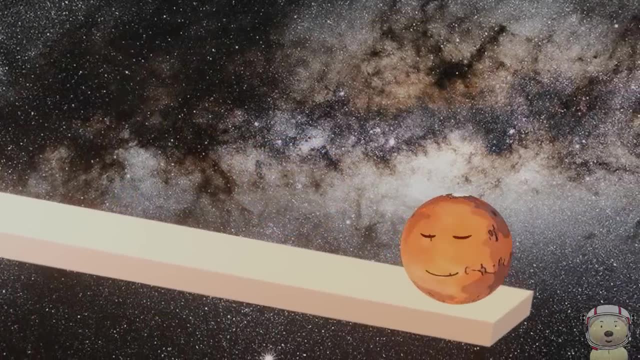 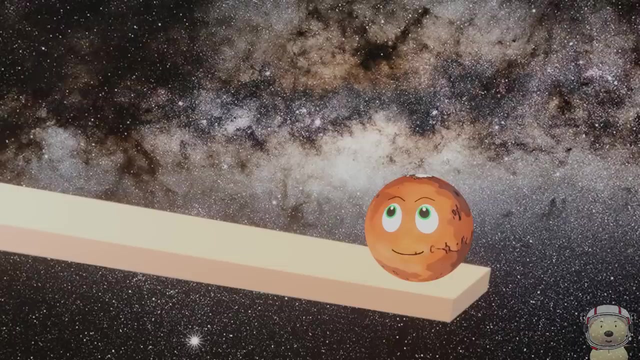 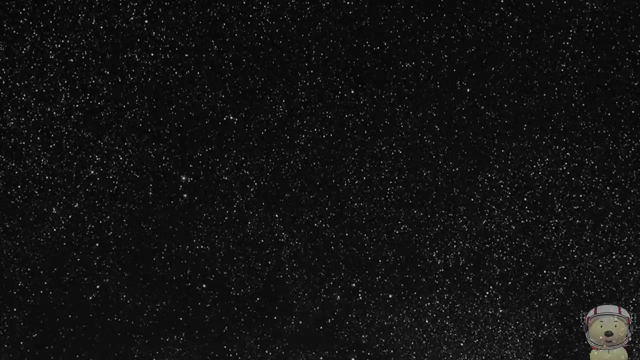 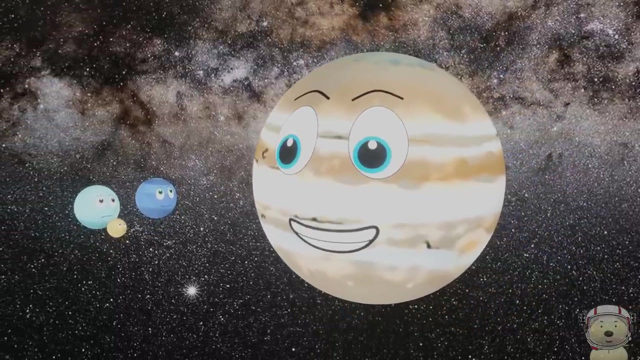 Yes, but just in case. Fine, But I am all that. you need Ready Jupiter, Are you sure? Mars, Yes, Let's go. Wheee, Hey, Big Jay, Hey guys, We are on our way to stop Earth playing computer games all day. 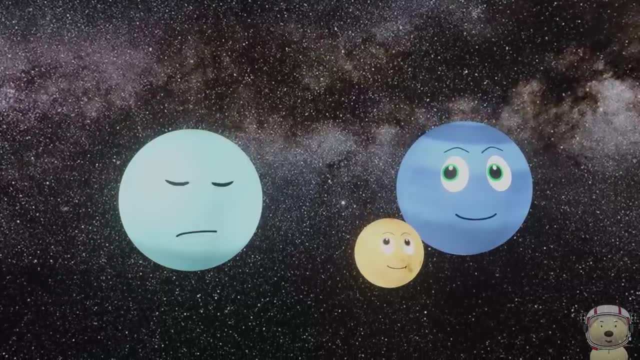 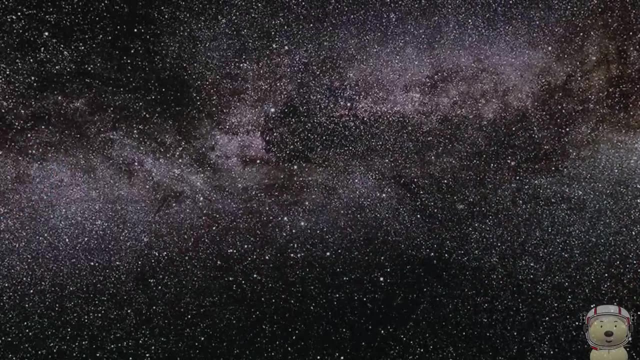 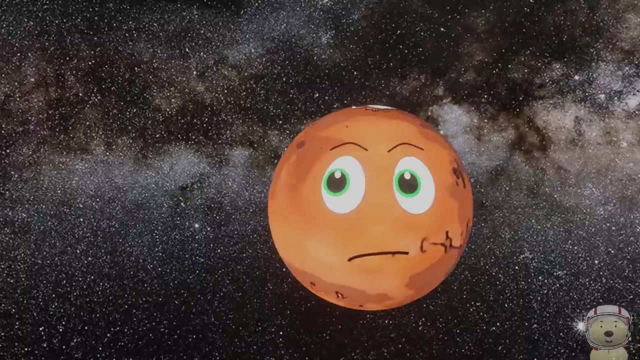 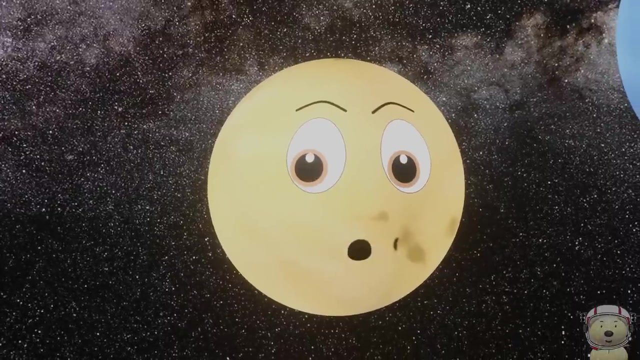 But I have such a good idea that we won't need you now. Wheee, Wheee. Can you help us out, please, guys? Yes, sure, Where's planet Uranus? I thought I saw him here. Do you guys know where Saturn is? 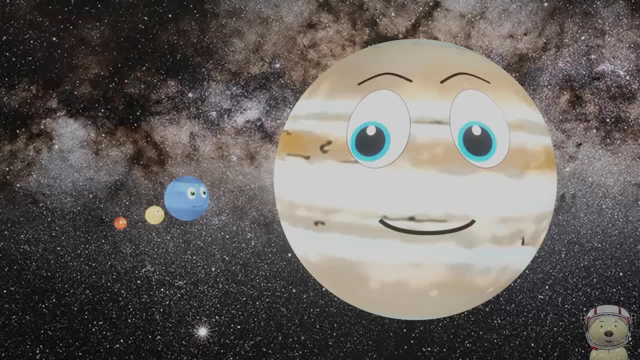 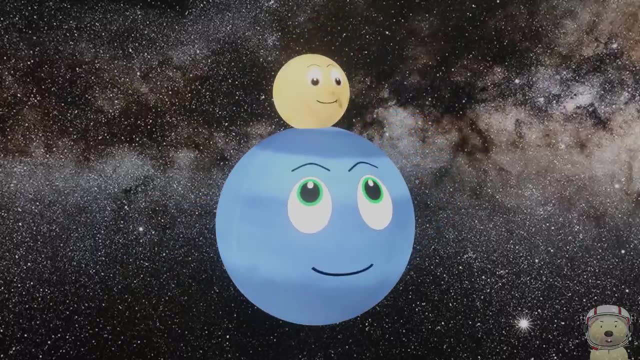 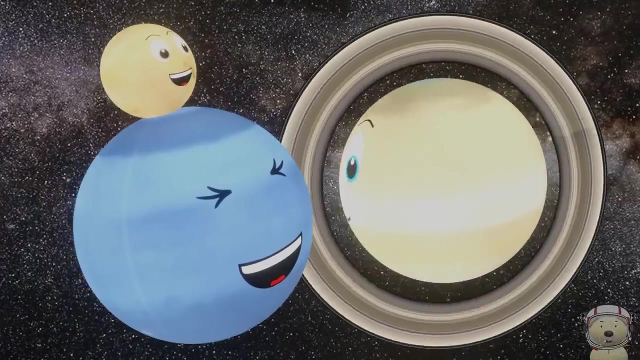 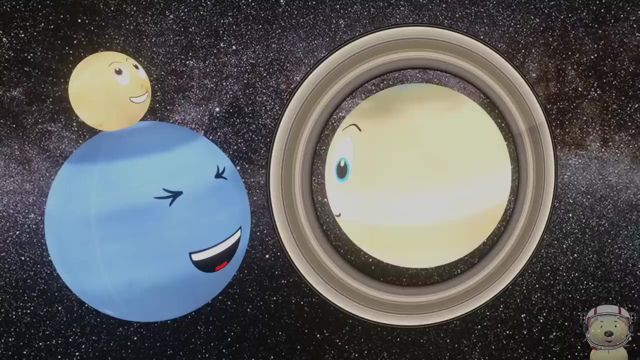 He's zooming around the solar system. You'll have to be quick to catch him. Hop on V, Use your strongest wings. Neck, Hey Saturn, Hey Venus, Nice wheels, dude, Thanks. Can you follow us to Earth's place? 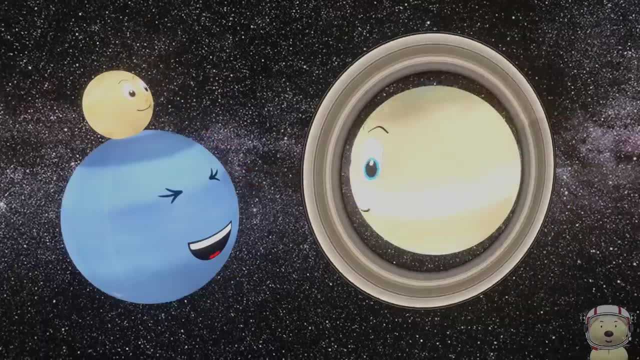 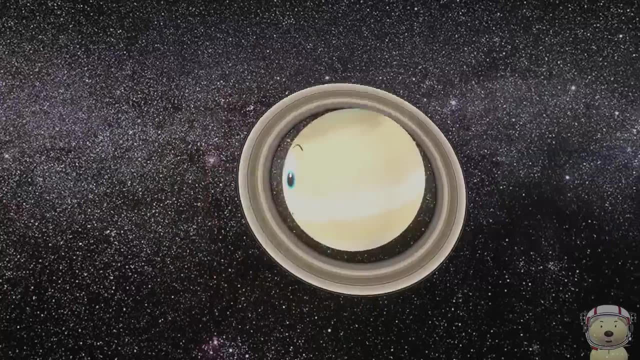 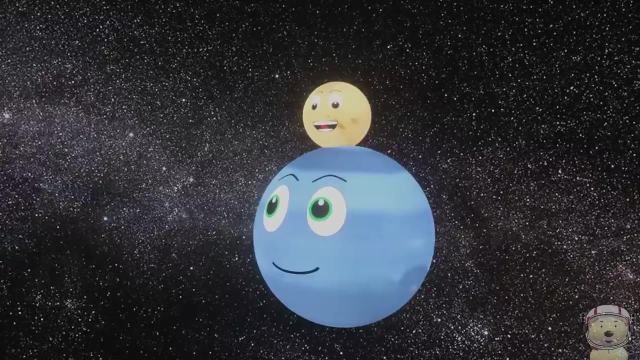 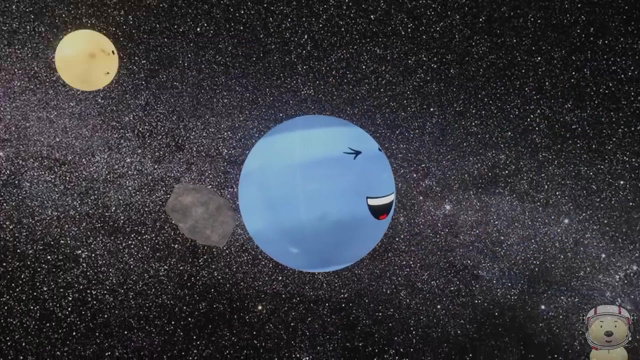 As his friends, we need to have words with him. Yes, sure, But before we go watch this Here, we go Watch this: Whoo-hoo. Think we can take it, Neck, We can make it Whoa. 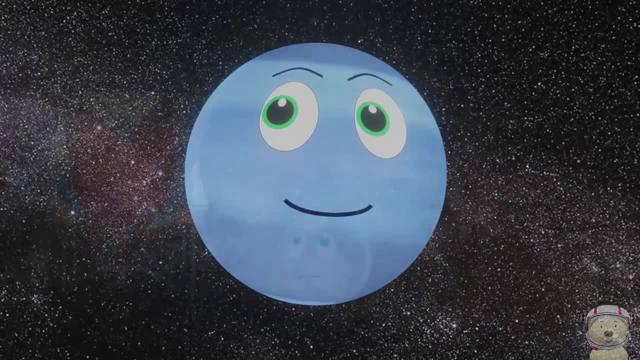 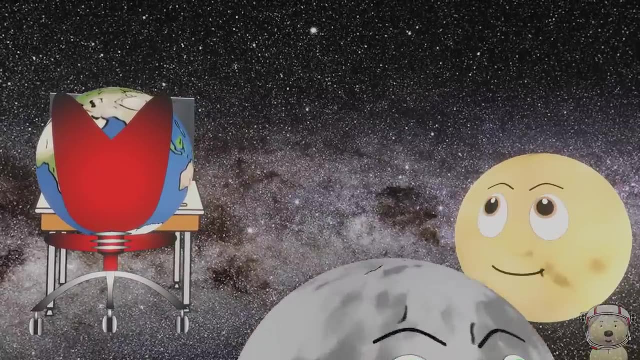 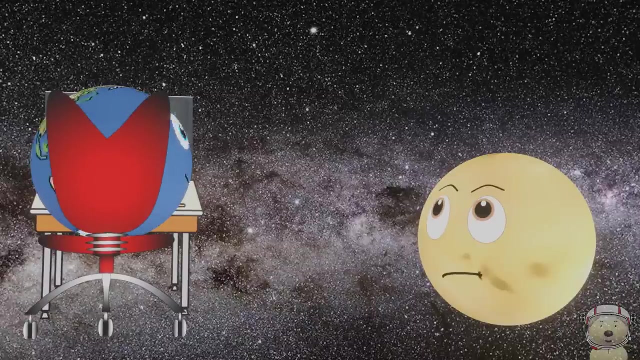 Er, nope, We can't make it. I can't get him off there. Venus, Thanks for trying. Mercury Earth, you need to come off now. No, Still playing, Can't See? Make way, dudes, Make way. 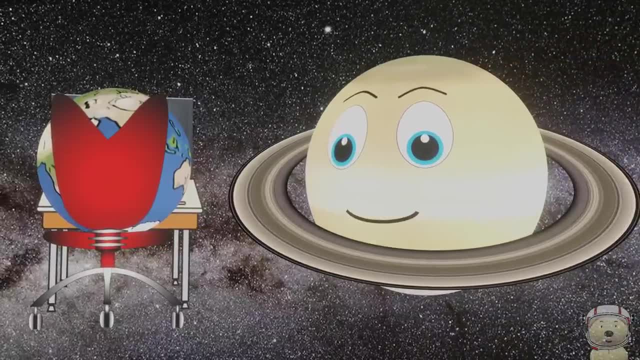 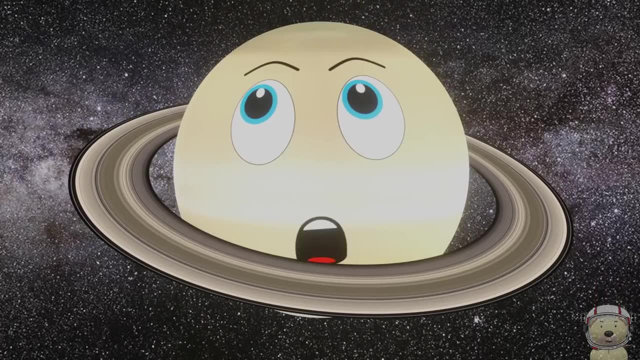 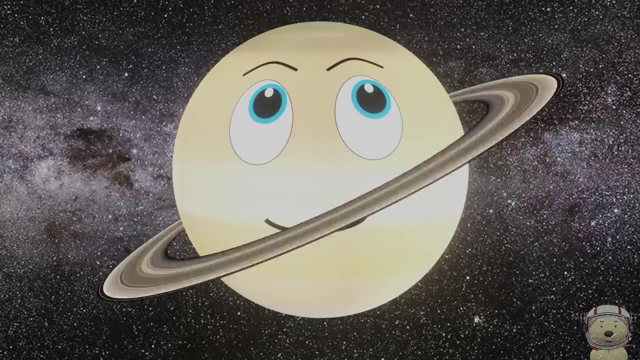 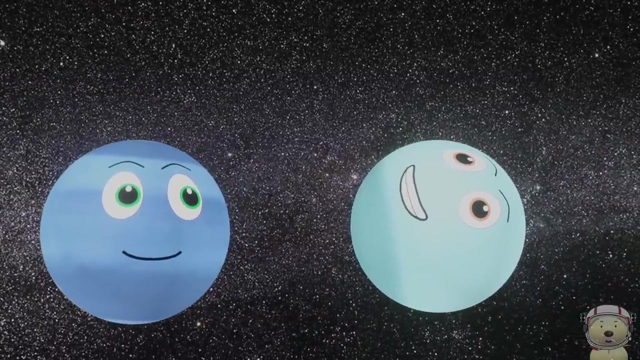 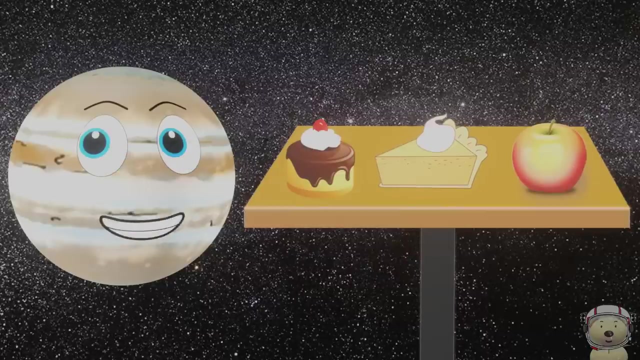 The secret is to entertain him. Watch this Earth dude Planet with the biggest ring system, Here we go. Oh yeah, All right. Oh no, Ew, for goodness sake, Cool, Look at these delicious treats- Earth. 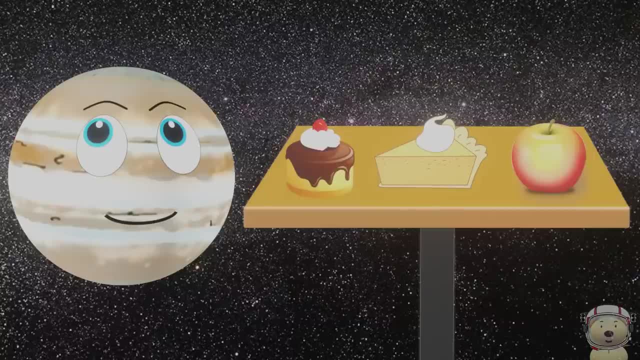 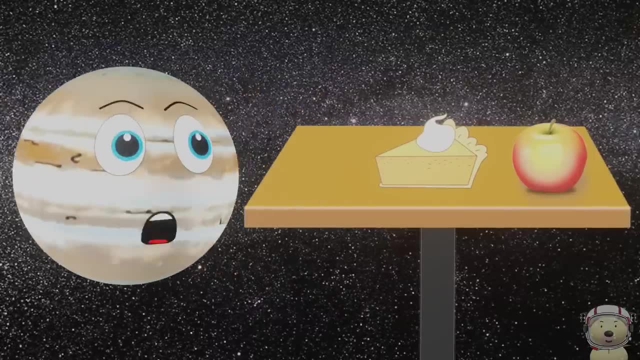 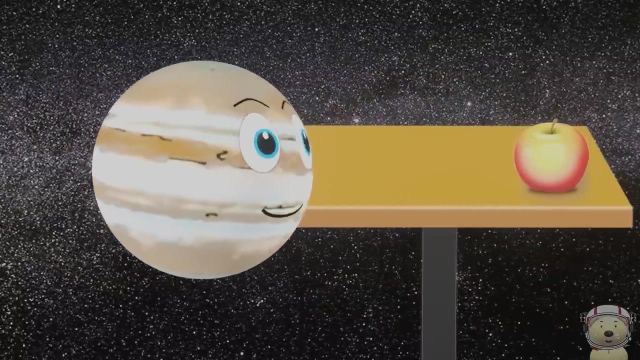 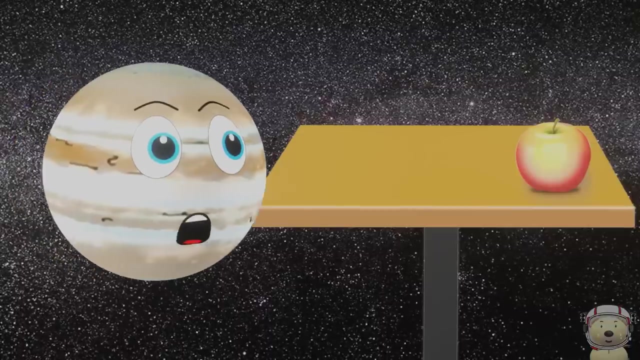 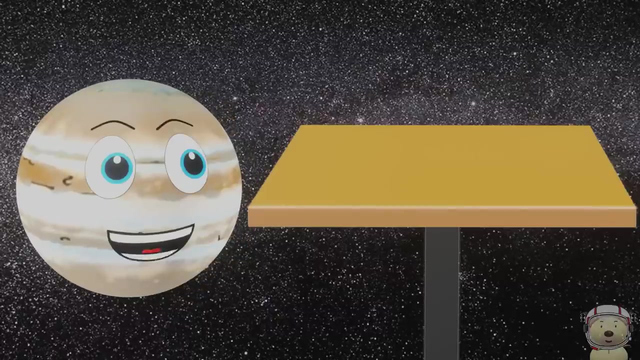 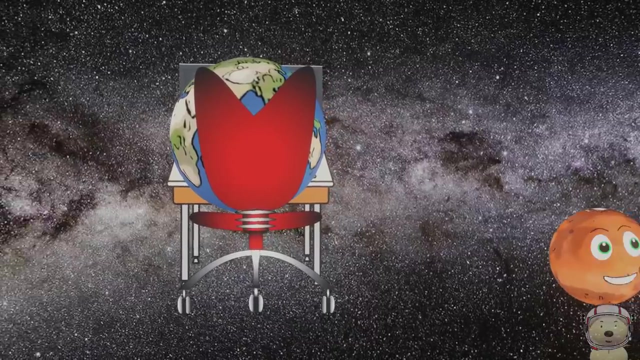 Being the biggest plant in the solar system makes me very hungry. Mmm- Delicious. Maybe one more. Mmm Beautiful. Yes, One more. I think Er whoops Brilliant. Let me sort this out. Watch this.